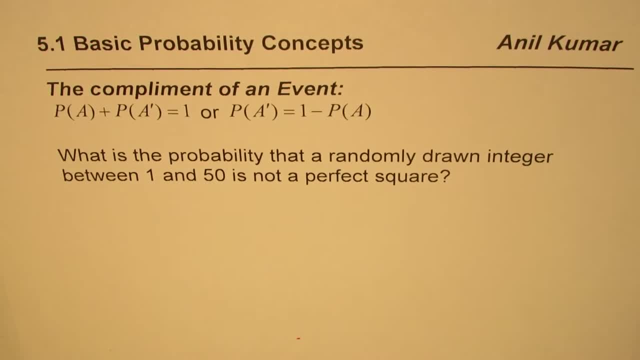 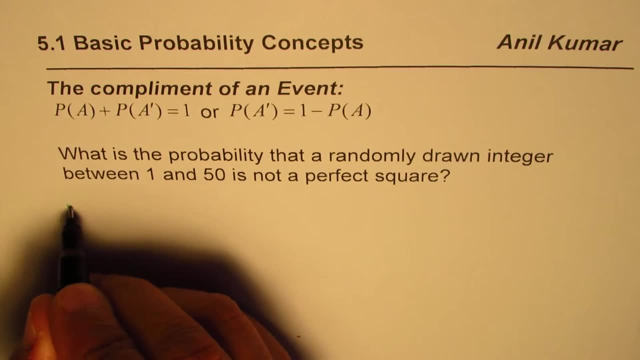 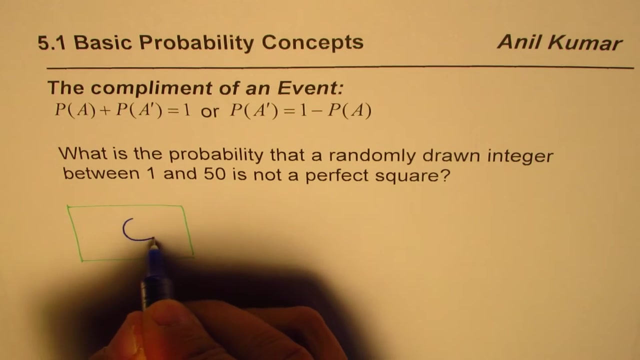 I'm Anil Kumar and in this video we will understand the importance of complement events. So normally in our sample space we are talking about a particular event of our interest. Let us say event A of our interest. is this event right? And the sample space is shown here. 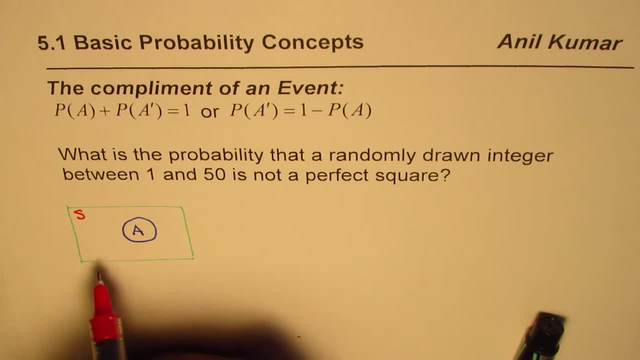 Then whatever is outside A is called complement of A right. So this part which is outside is A'. Sometimes you also write in different ways, right, Which could be kind of like this: okay, So what you observe here is that combination of these two is the whole sum of outputs or outcomes, right? 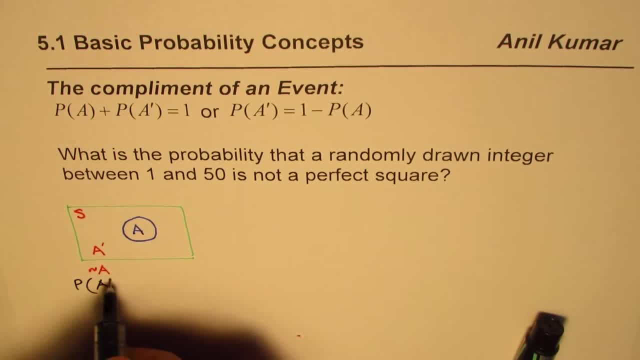 So the combination, So the combination of probability of A and the probability of A' or complement, is equal to 1.. So that is the concept which we can use to solve some questions. Here is an example: What is the probability that a randomly drawn integer between 1 to 50 is not a perfect square? 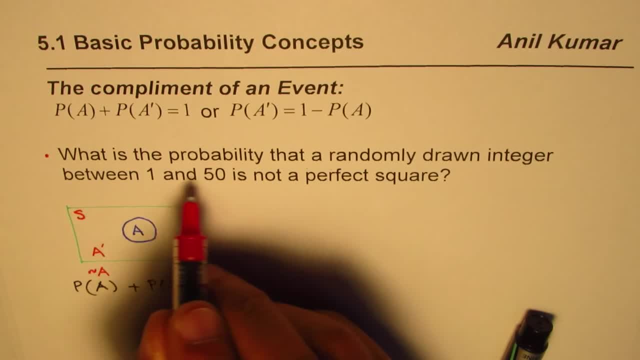 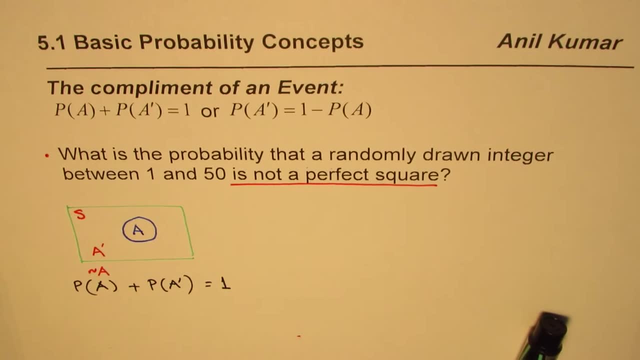 So we are saying we want to draw An integer between 1 to 50 and that should not be a perfect square. Now there are 50 numbers. Now which one of these are perfect squares? Let's list them Well first, what are all the possible outcomes when we draw one integer? 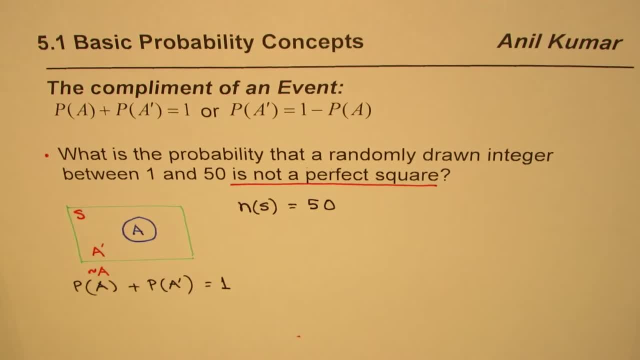 We have 50 as the possible outcomes. Now, how many of them are favorable? Now we say not perfect square. So there are a lot of numbers, but we can easily count those which are perfect squares. So let's think about those outcomes which are perfect squares. 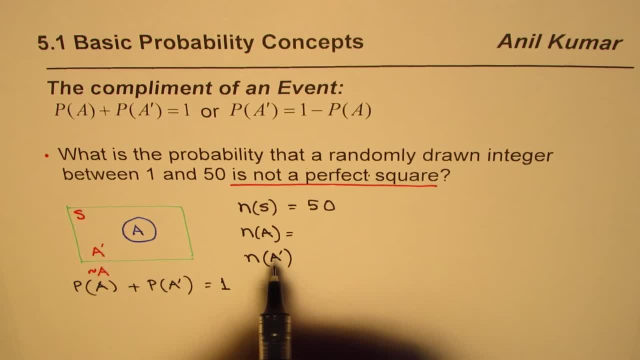 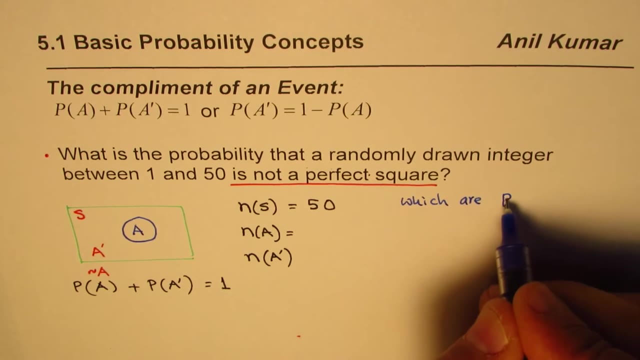 So when I say n of A', which is complement of our probability, that means we are looking for perfect squares in this case. So, out of these 50.. So, out of these 50 numbers which are perfect squares. So, out of these 50 numbers which are perfect squares. 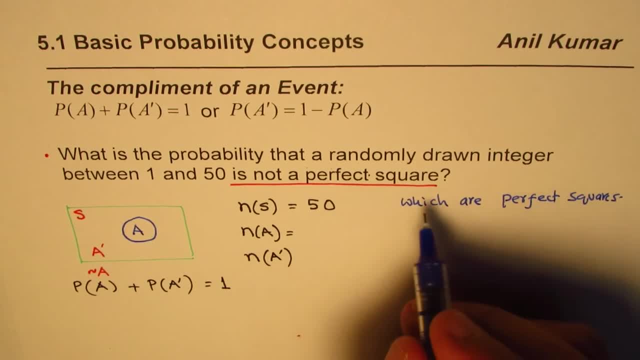 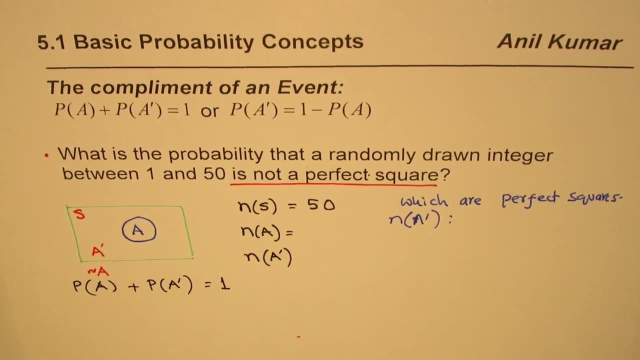 Okay, so that is complement to what we need. So that has been introduced to us as n of A' complement. right Now it's easy to find the perfect squares from the numbers 1 to 50.. For example, 1 squared. 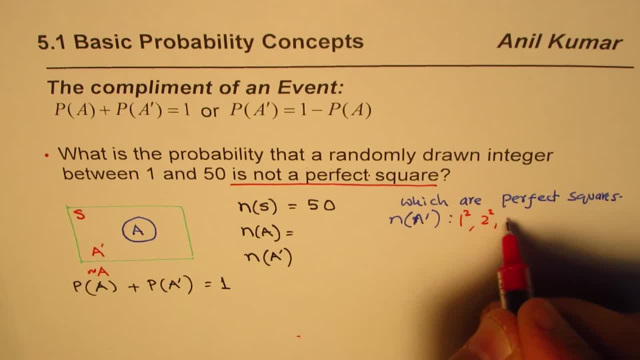 For example: 1 squared. For example: 1 squared: 1 squared is 1,, 2 squared is 4, 3 squared is 9,, 4 squared is 16,, 5 is 25,, 6 is 36,, 7 is 49, and 8 is 64, right. 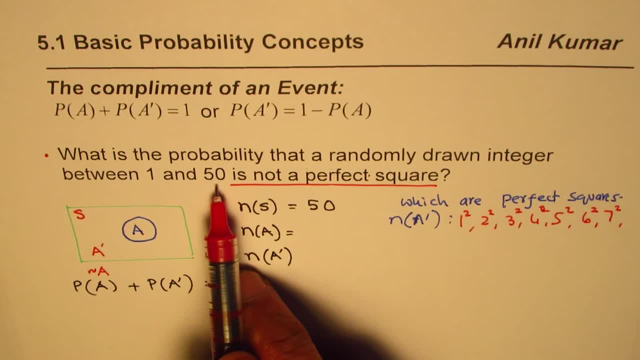 So straight away, we know 7 squared is 49,, which is less than 50.. So there are 1,, 2,, 3,, 4,, 5, 6, 7 perfect squares, Correct? So this gives you an idea that the complementary function, the number of outcomes which are favorable to perfect squares, is 7, right. 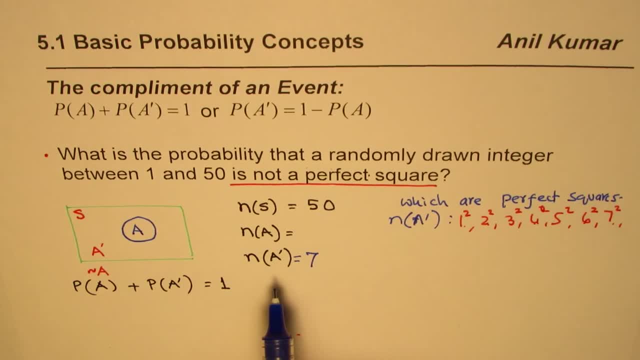 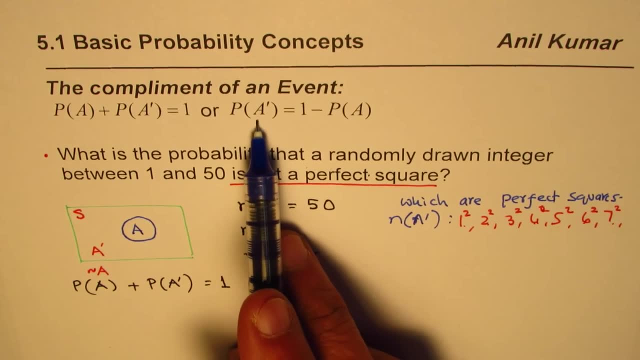 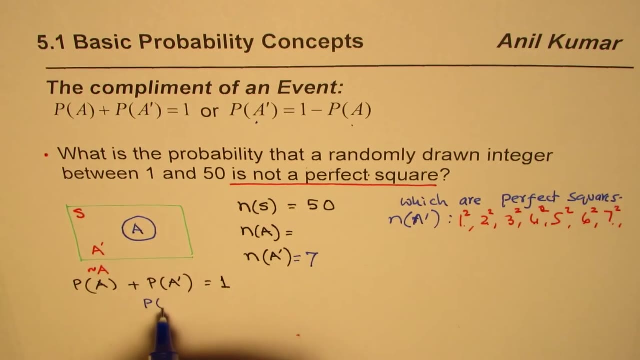 Now, if we find the probability of drawing a perfect square, then we can find its complement also using this formula, right? We know the sum of these two, We know the sum of these two, we know the sum of these two. So what is the probability of finding the complement? 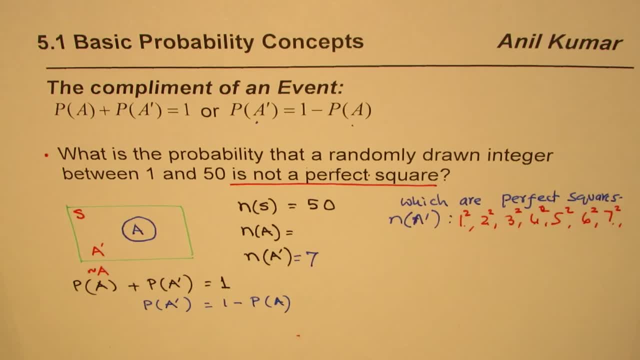 It will be 1 minus pA, right. So that is what we are kind of working on now. So what we are doing in this case is we find the complement. So in our case we have to find probability of A, we find the complement. 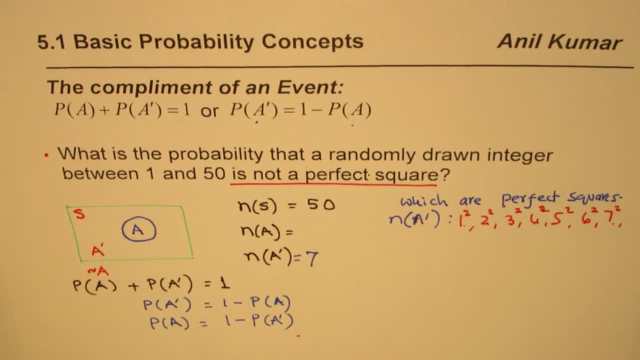 So we could write this as pA'. So either way, this formula can work. Correct, Correct, Correct, Correct. the probability of getting a perfect square, Probability of getting perfect square will be 7 out of 50, correct. Therefore, the probability of getting not a perfect square will be 1. 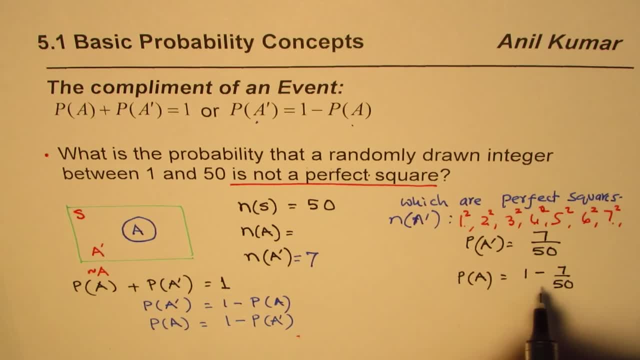 minus 7 over 50, correct. So that gives us the answer 50 minus 7,, which is 43, 43 over 50.. Is that okay? Now you could do it like this, or you could also do from here In our: